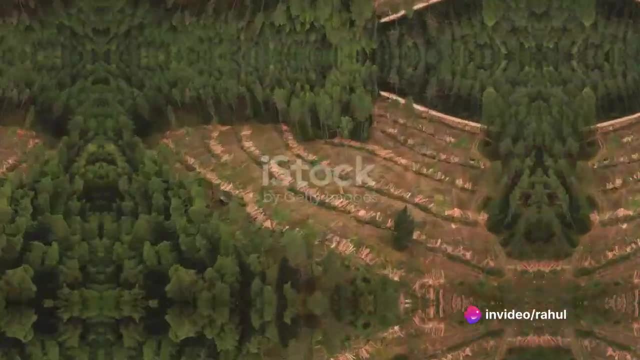 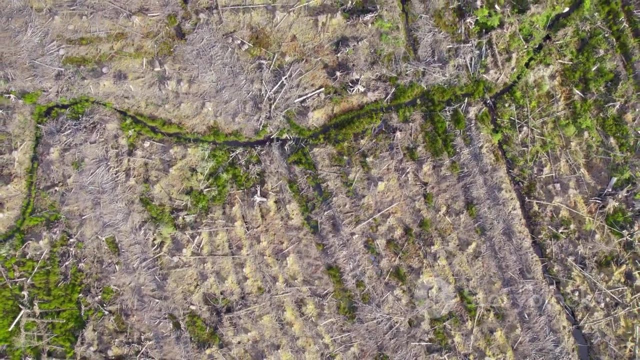 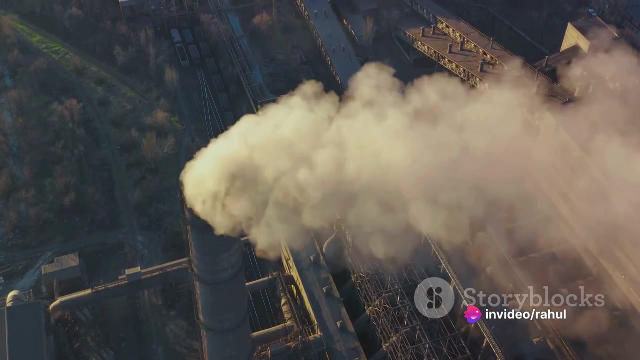 growth came a significant impact on our natural world. Forests that once stretched across vast landscapes fell victim to deforestation, Their lands cleared for agricultural purposes, logging and urban development. Industrial pollution from factories and vehicles tainted our air and water, creating a hostile environment for countless species, Species that once roamed. 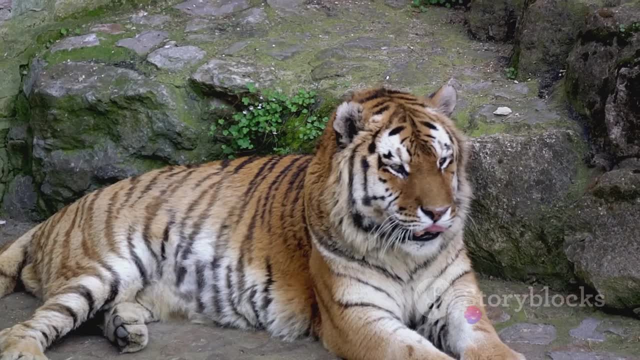 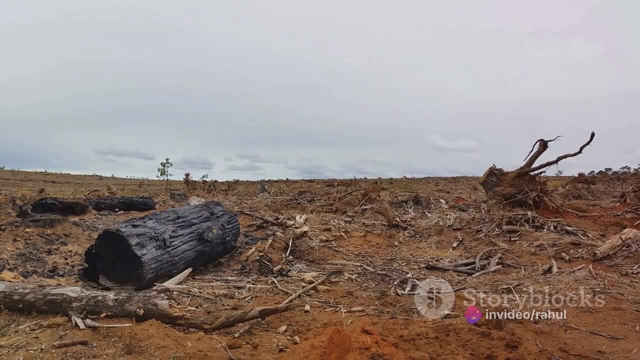 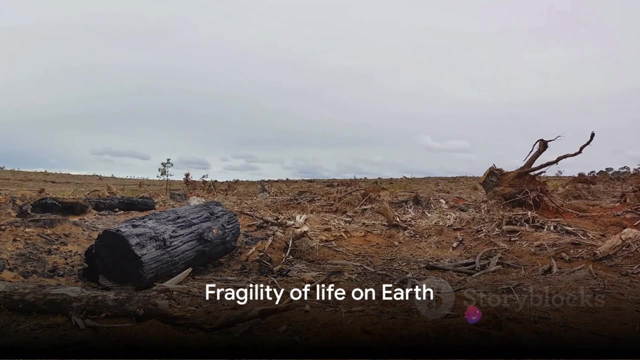 freely like the majestic Bengal tiger, the formidable African elephant and the magnificent blue whale found themselves on the brink of extinction. Habitat loss, poaching and human interference drove these icons of the wild towards a precipice. Their decline served as a stark reminder of the fragility of life on Earth. 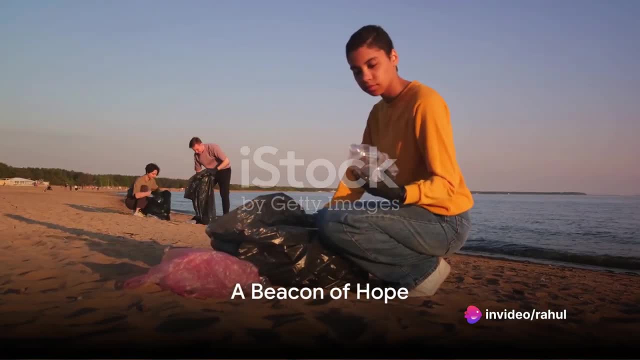 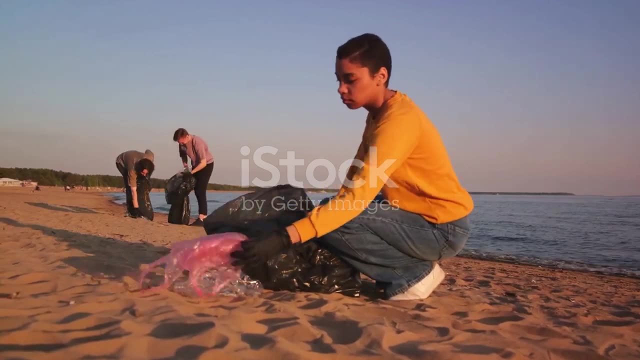 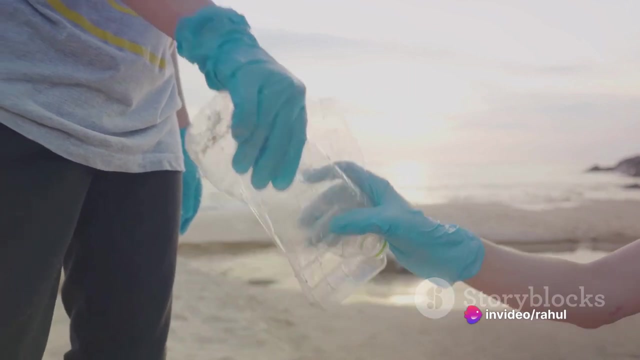 But even amidst this environmental devastation, a beacon of hope emerged. A worldwide movement advocating for conservation and sustainability began to take shape. Scientists, activists and local communities rallied together Their common goal: to protect endangered species, restore habitats and maintain ecological balance. With the rise of the 21st century, 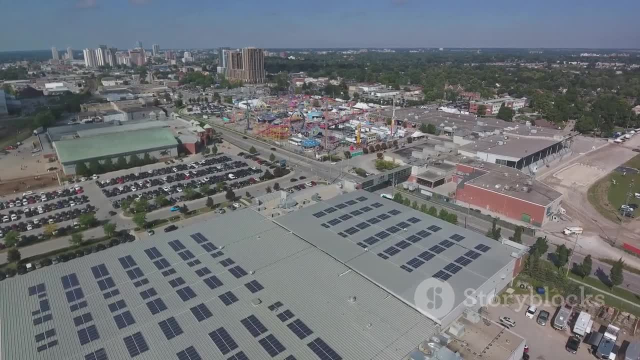 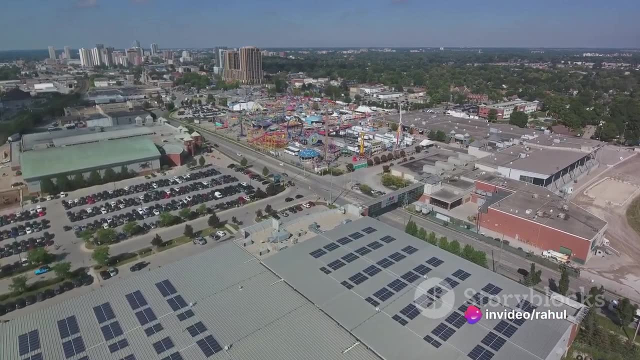 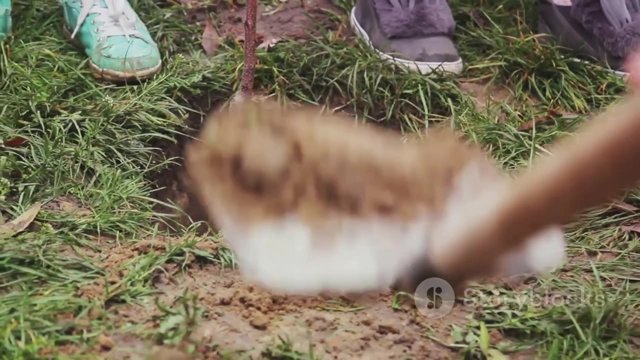 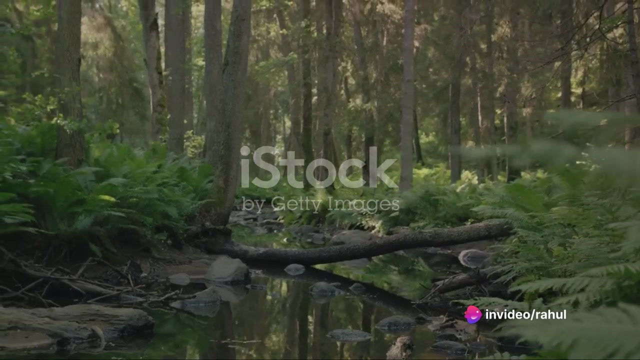 efforts to combat climate change gained traction. Initiatives aimed at reducing carbon emissions took center stage, Along with preserving biodiversity and promoting renewable energy sources. Fast forward to the present day and we can see signs of hope. Nature is beginning to reclaim lost ground. Landscapes once stripped bare are now lush with reforestation efforts. 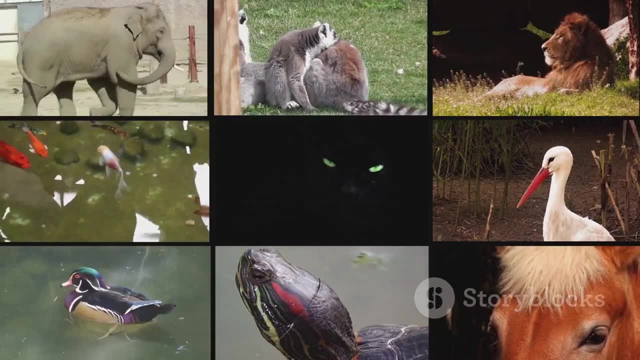 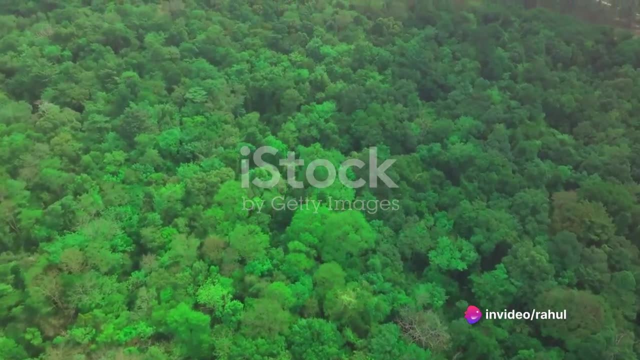 Species that teetered on the brink of extinction are making remarkable recoveries. In reflecting on the past hundred years of change, it becomes clear that the fate of our planet is firmly in our hands. By embracing and prioritizing conservation, sustainability and stewardship, we can ensure 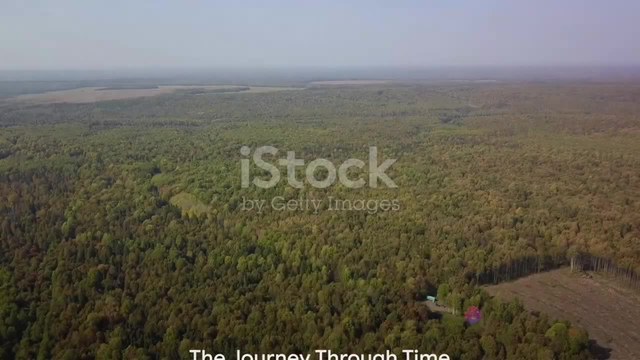 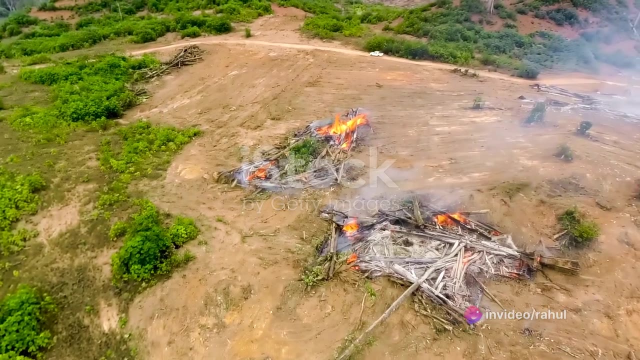 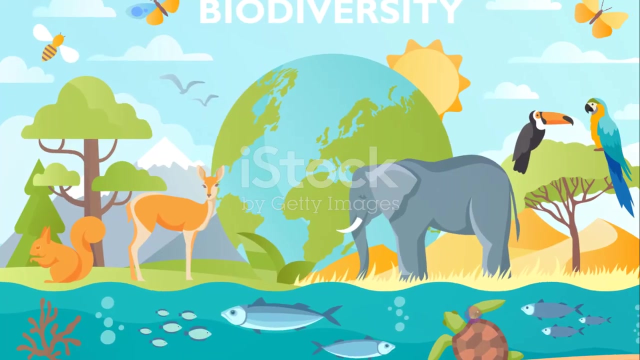 a brighter, healthier future for the generations that follow. In examining the past century, we've journeyed from the dawn of the 20th century and the emergence of industrialization, through the devastating impacts of deforestation and pollution, to the rise of a global conservation movement. We've seen the decline and resurgence of species. 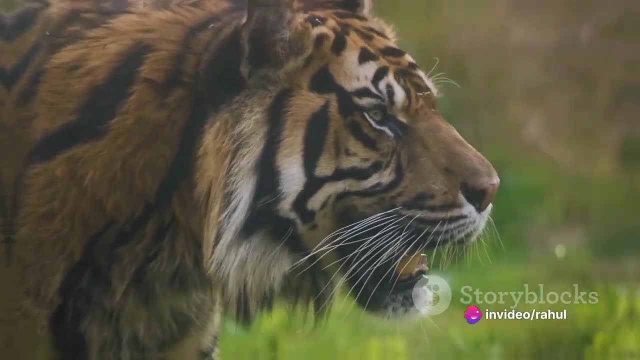 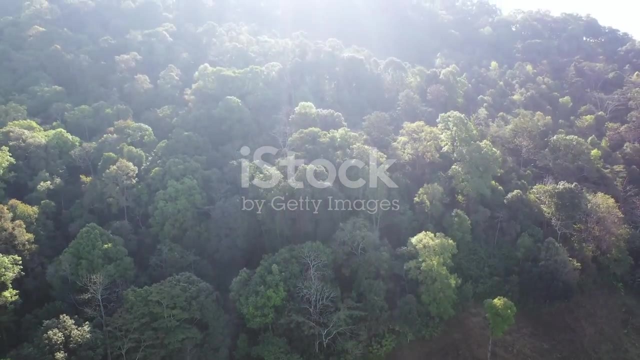 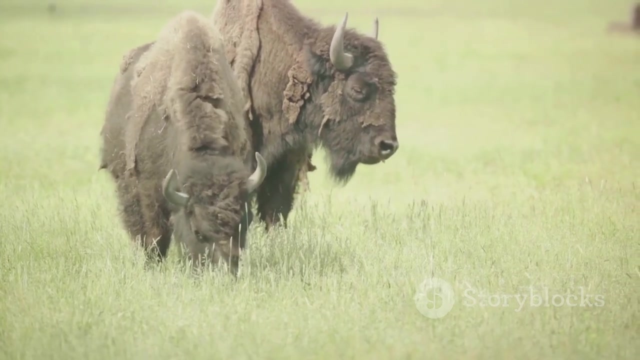 and witnessed the transformative power of sustainability efforts, And so we end our journey here with a glimpse of what the future can hold if we continue to respect and protect our planet. This is the story of a century of change, global flora and fauna, a testament to the